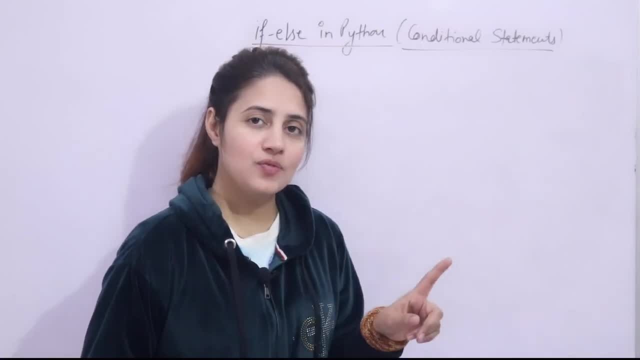 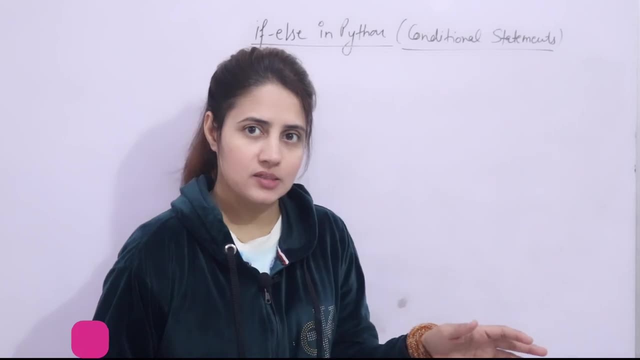 So in the series of learning Python programming language, in the previous video we have seen one coding exercise, like in weeks, and we have discussed what are f string and based on that we have seen that exercise right. So now in this video we will talk about if statement. 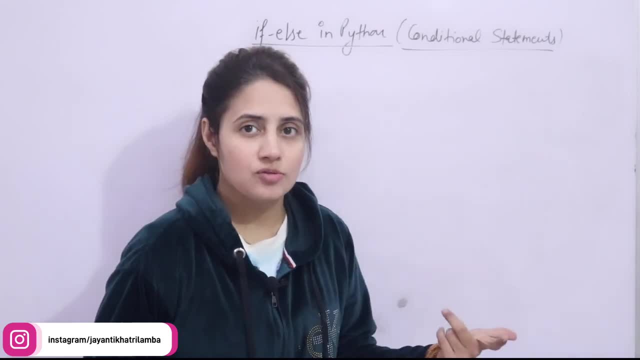 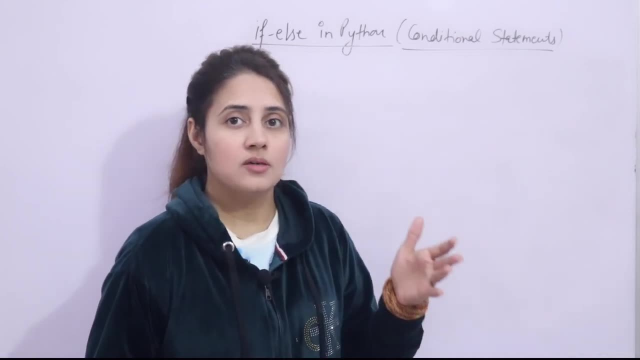 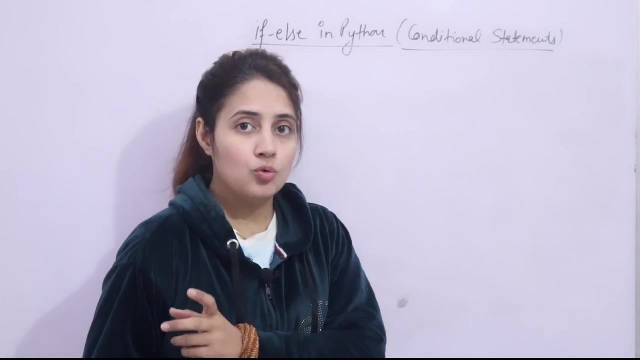 and if else statement. in Python These are known as conditional statements, control statements also. we can say decision making statements Simple: if, if else nested, if else else if. whether these are decision making statements, right Or conditional statements, So one. 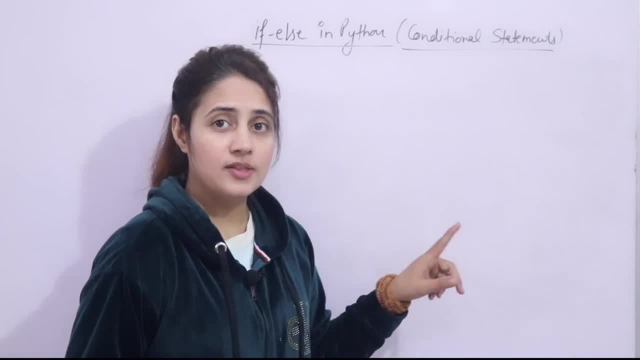 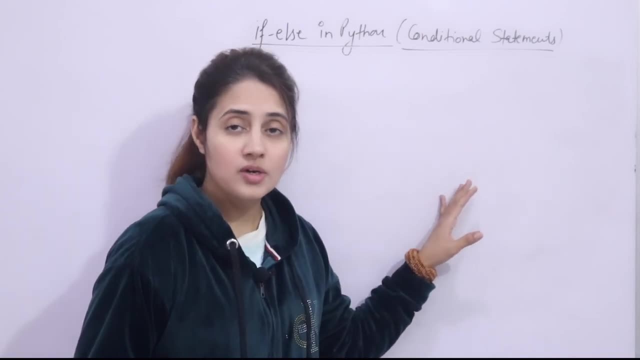 by one. we will be discussing these statements and this video will talk about if and if else, with the help of real life example, as well as with the help of program, the syntax, when we should use if else, when we should use if statement. all the things we will be discussing. 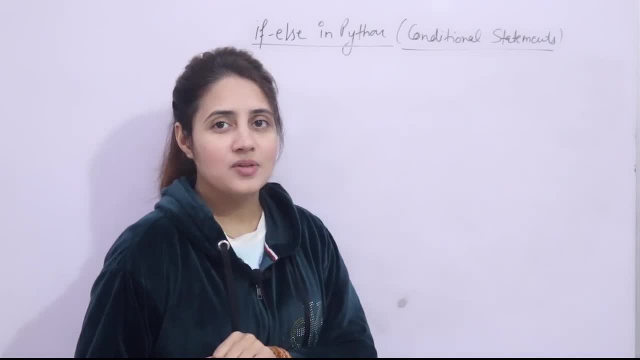 in this video right Now. before that, I just want to tell you one thing. See, the journey towards becoming a PSU officer or pursuing MTech from IIT or other elite institute is going to be long and challenging. So for you to understand this video, please do subscribe to my YouTube channel and hit. the bell icon And if you are new to this channel, please do subscribe to my YouTube channel. If you are new to this channel, please do subscribe to my YouTube channel and hit the bell icon, And if you are new to this channel, please do subscribe to my YouTube channel. 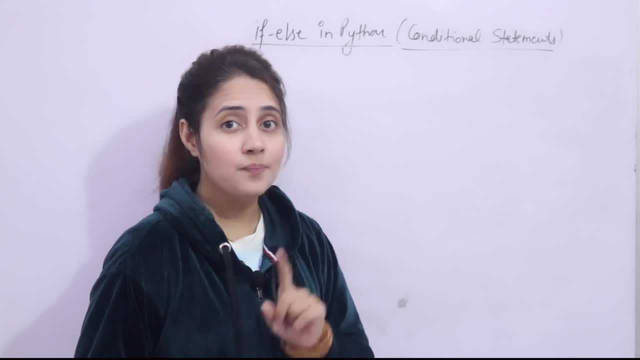 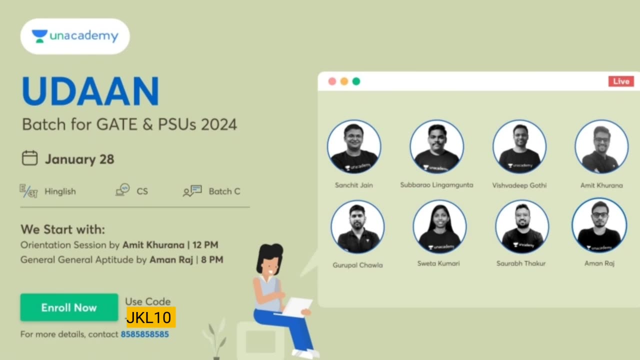 To start you, to stay focused on your path. Here are some confidence booster initiative by an academy, and academy is going to start udahn by batch four, gate 2024 aspirant and five aspirants. So here and academy stop. educators will be teaching you in these batches And 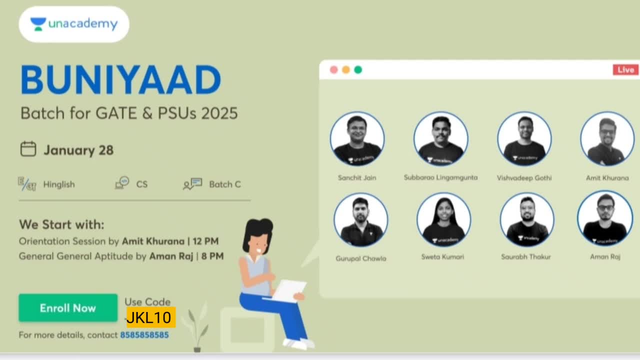 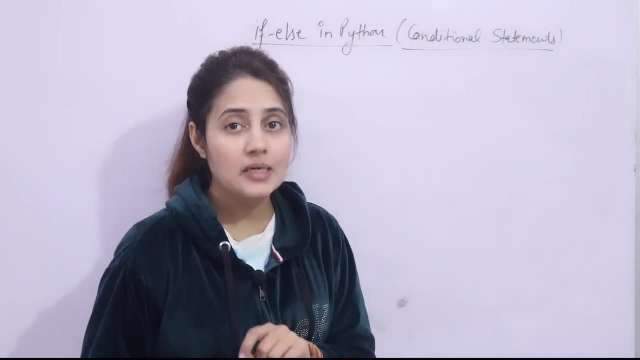 these batches will be in English language, both in the conventions, But if you want to attend lectures in complete English language, then for you also. they have started a batch Ignite to point zero four, gate twenty twenty four, aspirant and Foundation for. 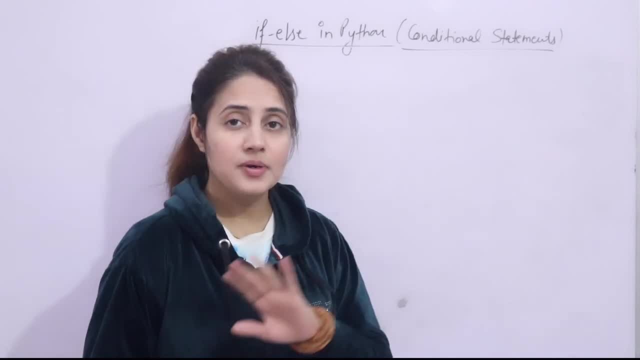 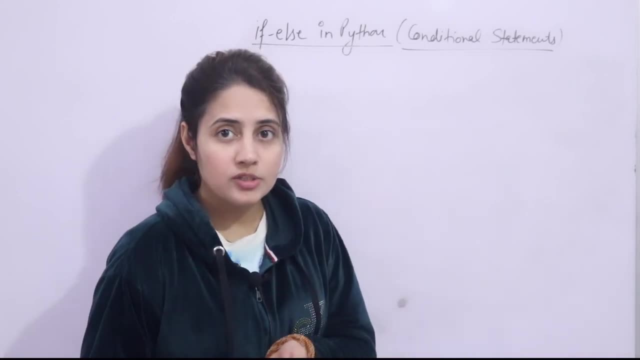 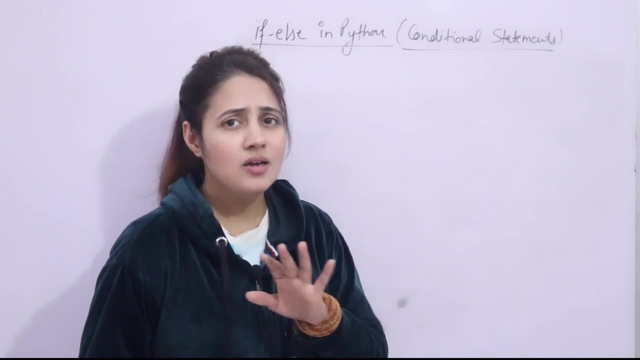 GATE 2025 aspirants. In these batches you will get comprehensive syllabus coverage, PSU exam preparation, interview preparation, previous year questions plus daily practice question and digital books, home delivered printed books, practice question of you know, practice of test series and much more. and one more thing on this republic day. 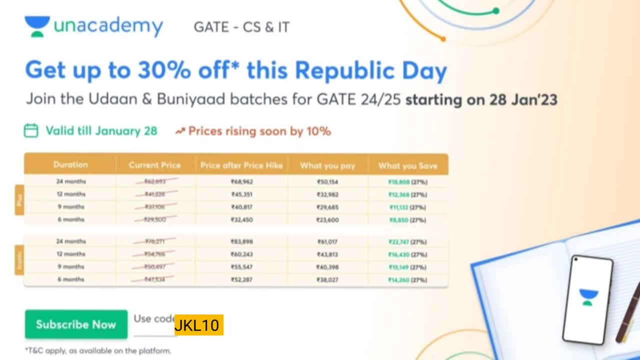 an academy is also, you know, providing you some offers. If you take plus or iconic subscription of GATE and ESE, you can save up to 30 percent. Yes, you can see on my screen here the price detail, but this offer is valid till 28th of January. and remember one thing: there will be price hike soon. 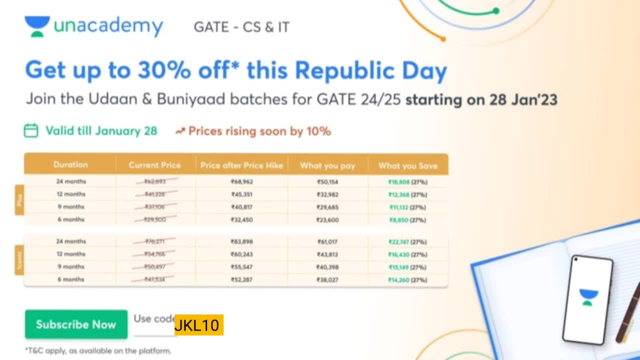 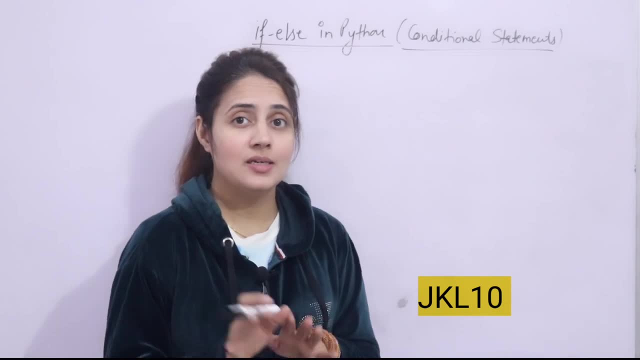 for this subscription. So do not wait and subscribe today and start your GATE and ESE preparation. and to avail these discounts, use my code JKL10.. So all the relevant links and details you will get in the description box of this video. you can go and check out. Now let's see what are. what are? 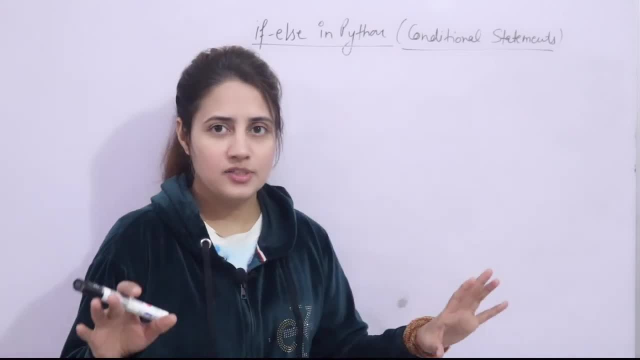 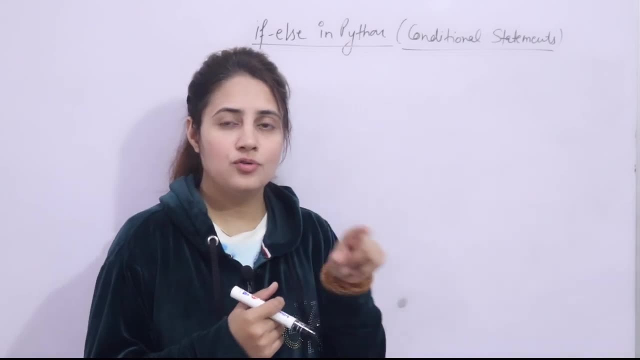 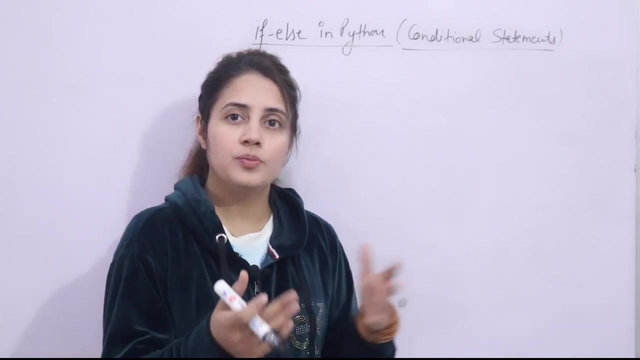 this efforts and if statement in python. see, let's take one real life example. whenever you go to, generally, you travel in metro. so there is a board like: if your child height is less than three feet, then no token required, right, you don't need to purchase any token or ticket, anything right. but if height 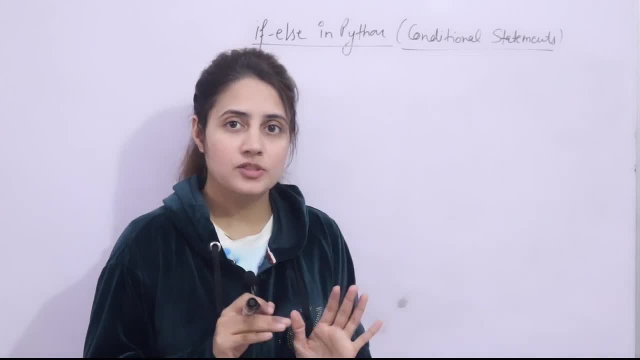 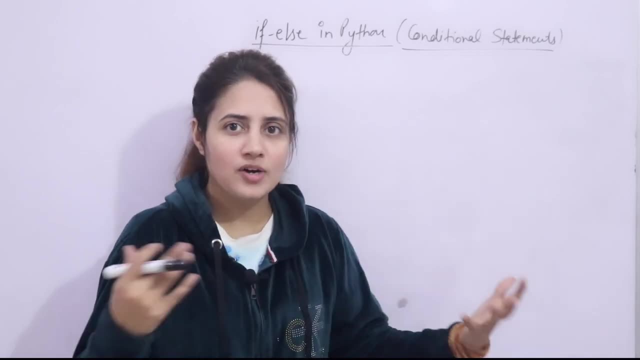 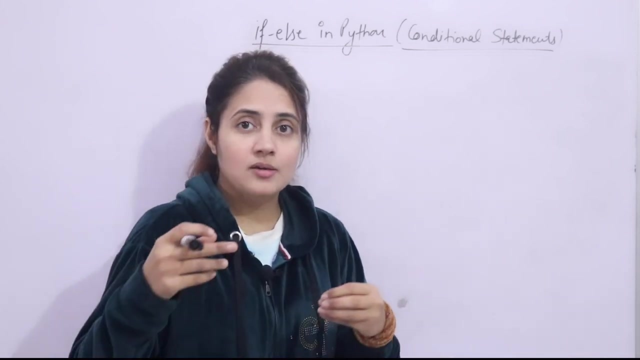 is more than three feet three feet, then you have to purchase token. so there is some condition right in a real life also. everyday we are facing these type of conditions and based on some condition we take decisions right. like if you go to supermarket and your mom say please bring some. 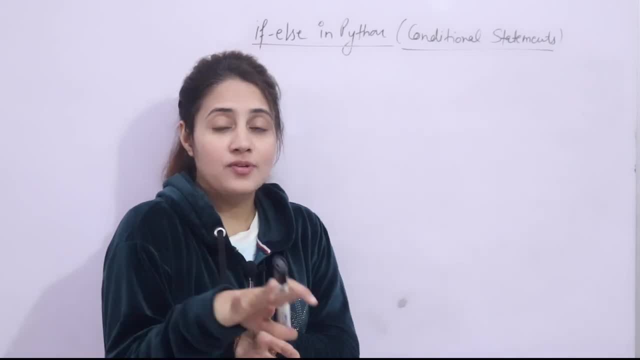 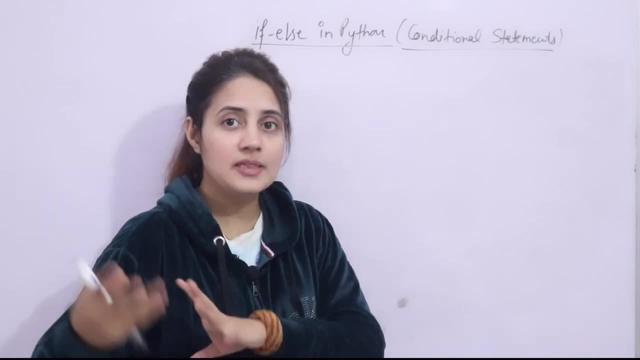 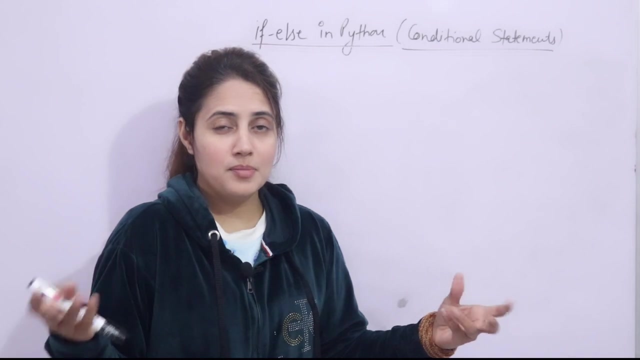 you can say: buy some apple. maybe you will ask: if apples are not available, then what should I buy? then maybe oranges, and if oranges are not available, then maybe dragon fruit. so there also you have to decide, like maybe you are a coffee lover or, but based on your pocket money, you will have coffee. 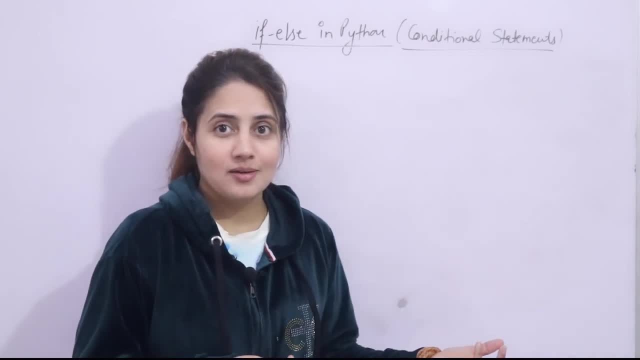 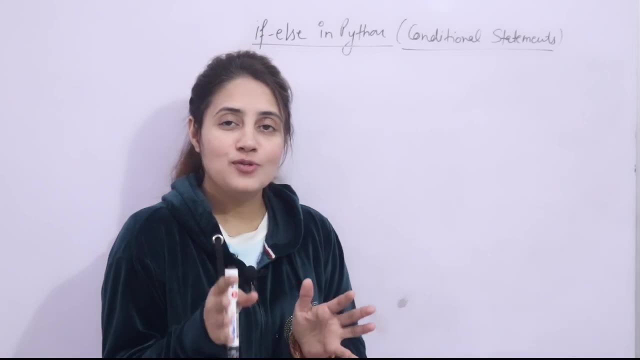 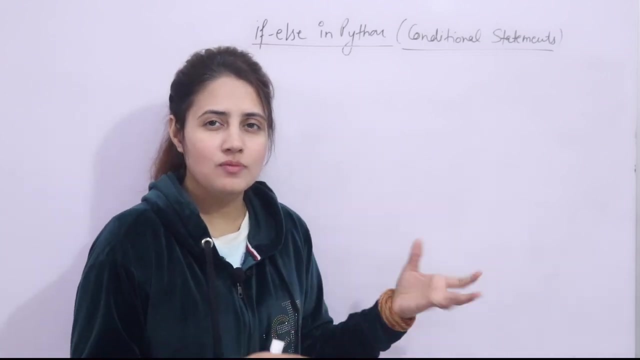 maybe in starbucks or at some store, now that that decision is based on your pocket money, right, how much money you have. so in real life also, we are taking multiple. you know many decisions every day, so when we write program, then also obviously we will. maybe we are working on a project, we'll 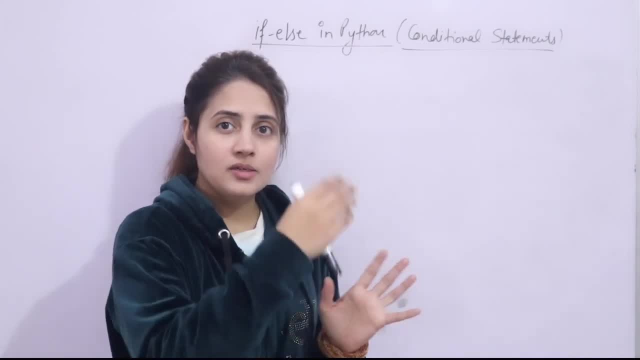 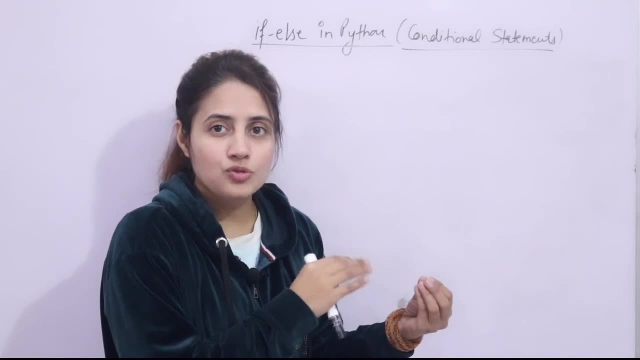 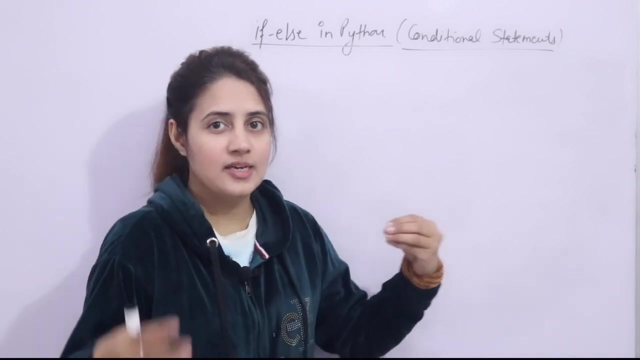 create some product and all. so to map these decision making, these things in programming, how you can write down these things. so, for those we have conditional statements using if else, using elif, using, you know, multiple, if else nested, if else else, if ladder, we can map these decisions. we. 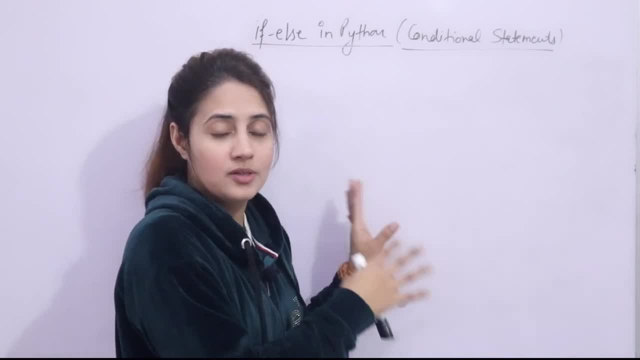 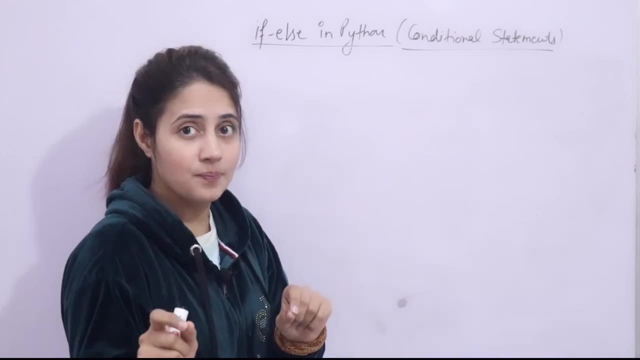 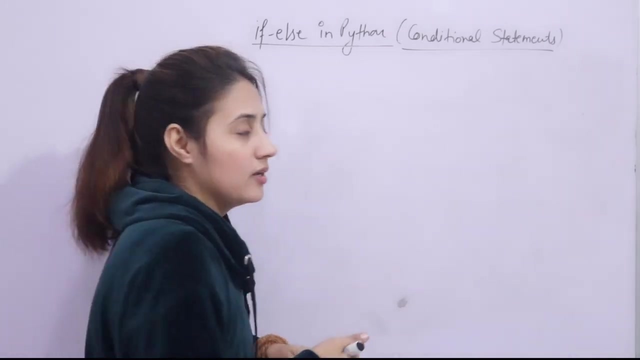 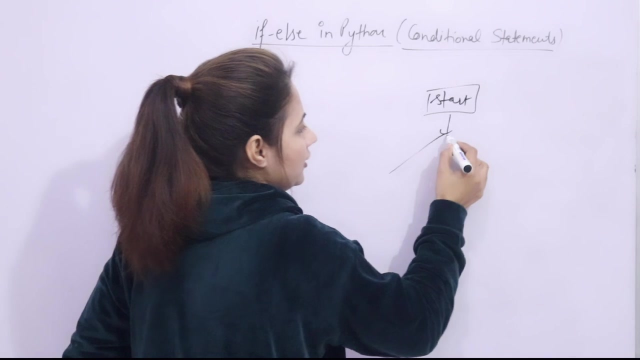 can write down these decisions in our programming, in program, in the form of programs, right? so that is why these are known as conditional statements, or you can say decision making statements. fine, now that that let's take that, that example, that height, height of your child. so if I like, if I draw a flow chart, then obviously start, and here we have a condition: height height is greater than 3.5. 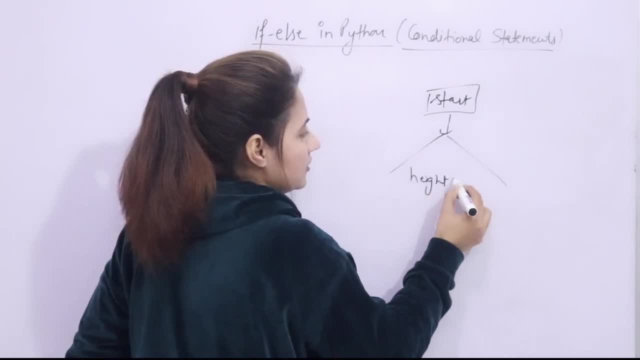 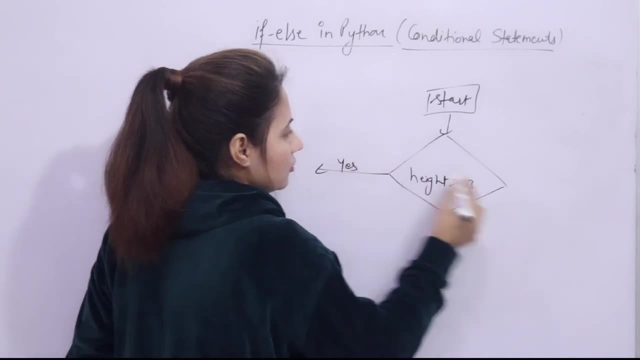 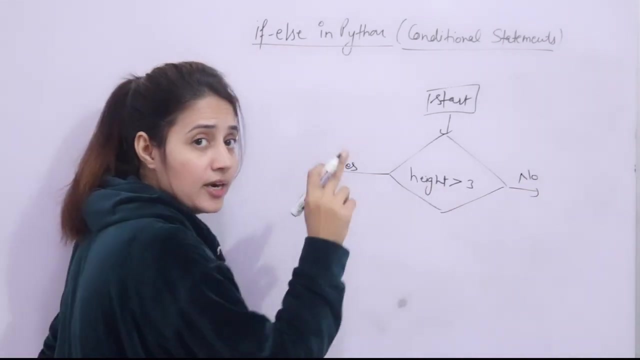 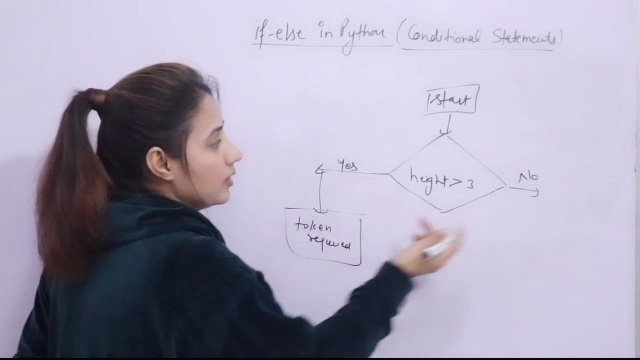 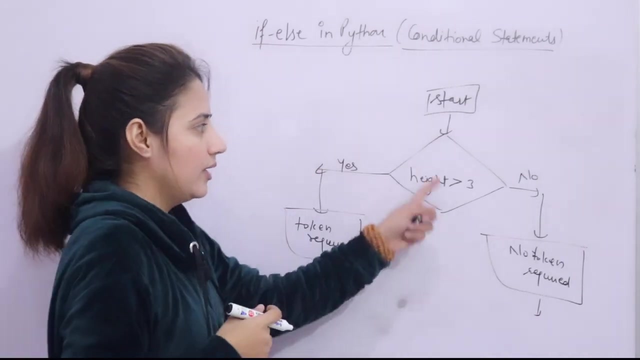 height. height is greater than 3.5. than three fit. I am taking height, I am taking in fit. two condition can be there: yes, your child height is greater than three or not, or no. if yes, height is greater than three fit, then token required to board metro. if no, then no token required. so this is how we can, like we can, you know, draw a flow chart. 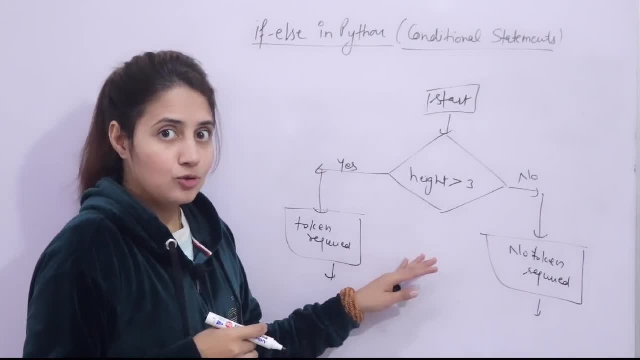 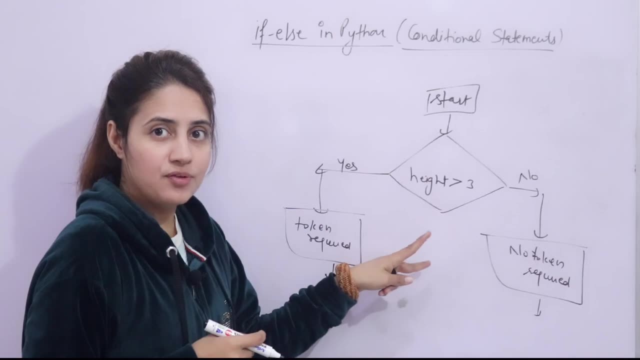 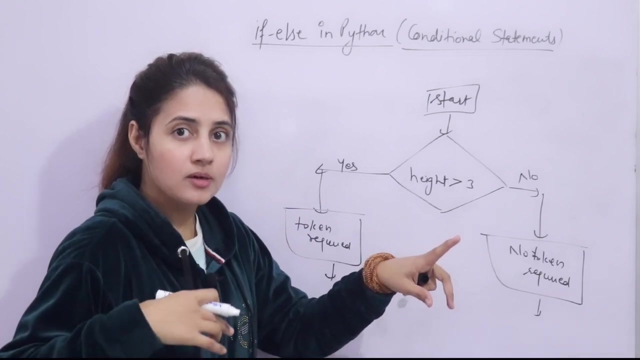 kind of thing. right, this is the case. so to map this thing in program, what we will write? if else? because here we have two choices: yes or no. so if or else, if apples are there in supermarket, buy apples, buy apples, otherwise buy oranges. two choices you have. 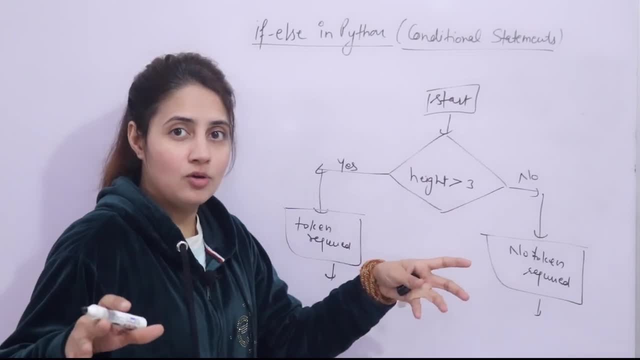 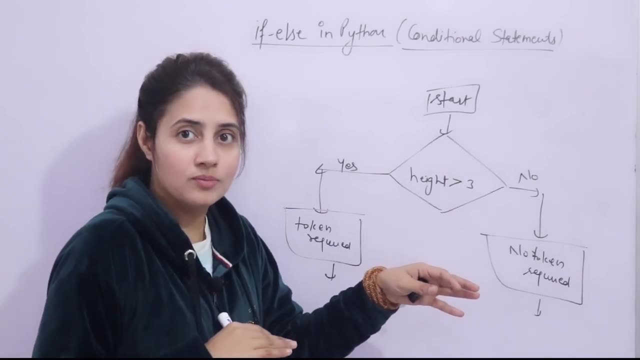 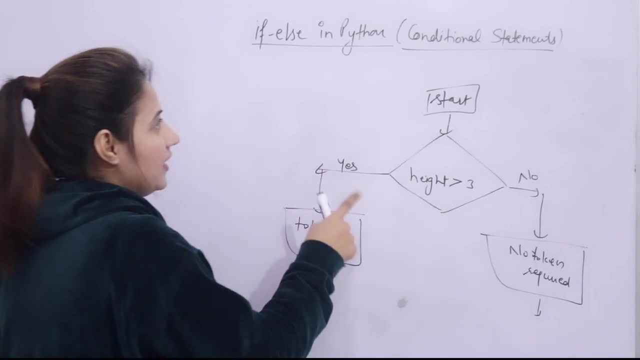 right if there is only one choice. maybe your mom say: if, then buy apples, otherwise nothing back to your own, come back so that we can write with simple if no else required. but here we have two choices. so if and else. right now, what is this general syntax of writing? if simple, we will. 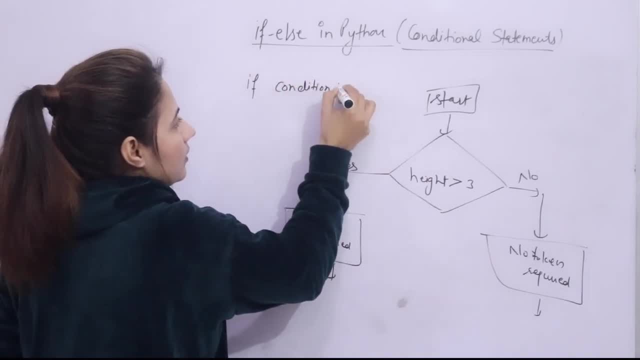 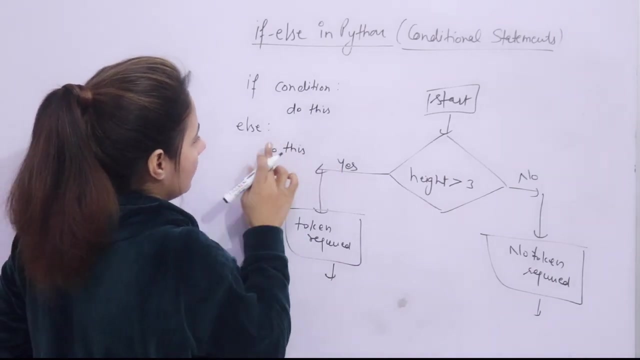 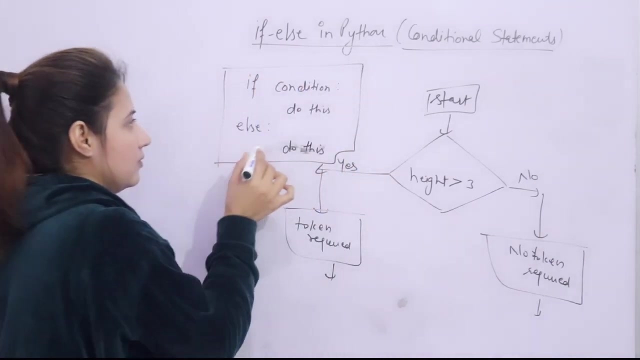 write if- and here some condition, then colon, then the block of statement that should be executed. if this condition is true, that would be here. we can write down like: do this else, colon, do this right. see, let me just tell you one thing. one thing is very, very, very important. when you write if else in Python, or when 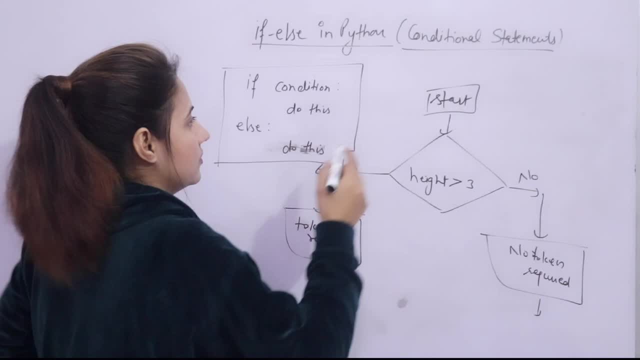 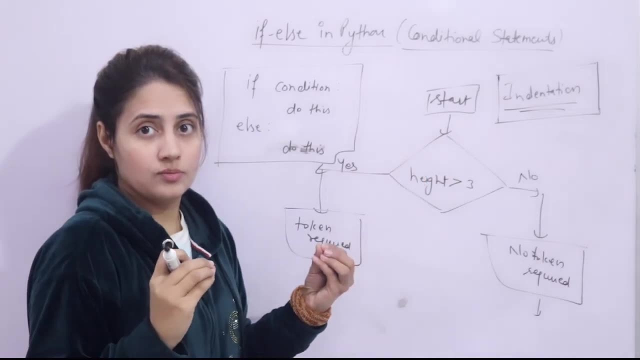 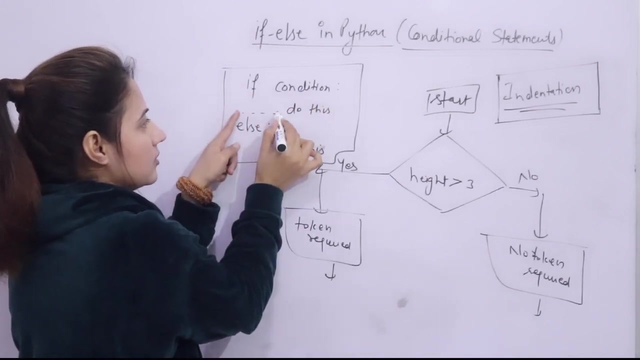 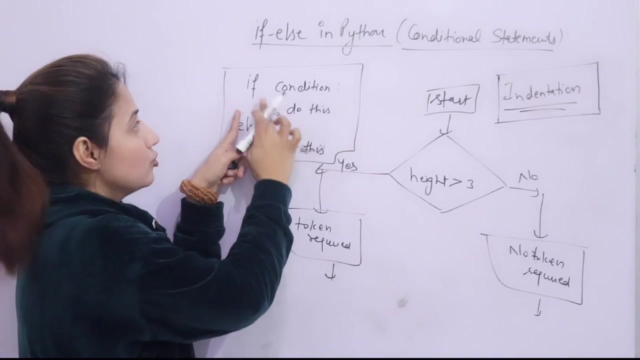 you write programming in Python, that is indentation, because Python basically use indentation to identify a block. what is this indentation like? if you write this statement, then, after some space, this space before you know, in the beginning of this line, this is known as indentation, right? so if we write: 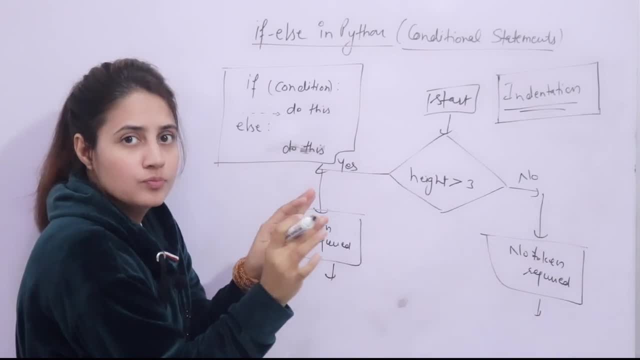 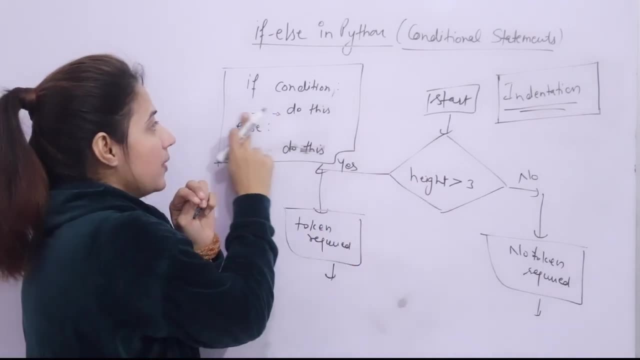 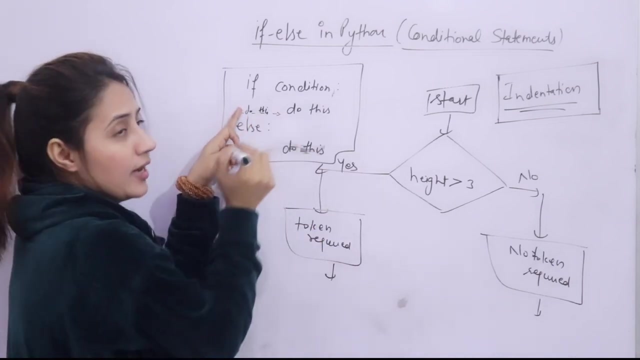 condition, condition you can write down in these brackets also. or if you do not put these brackets, that is also fine in Python, right? both the cases are true. but this space, this indentation is must directly. you cannot write down from here. do this, that will give you error. 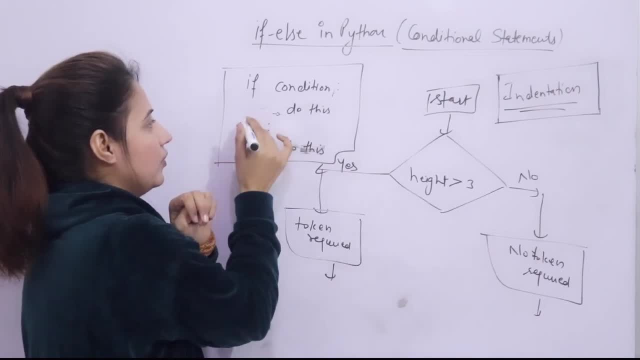 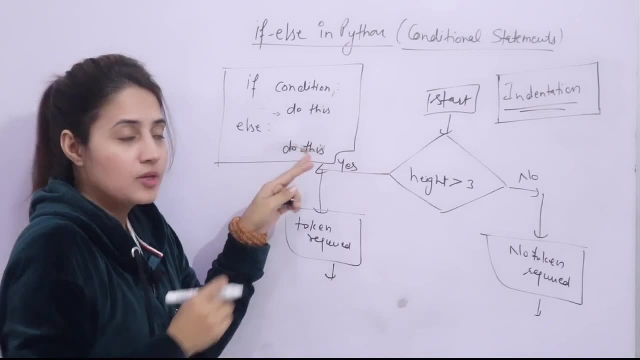 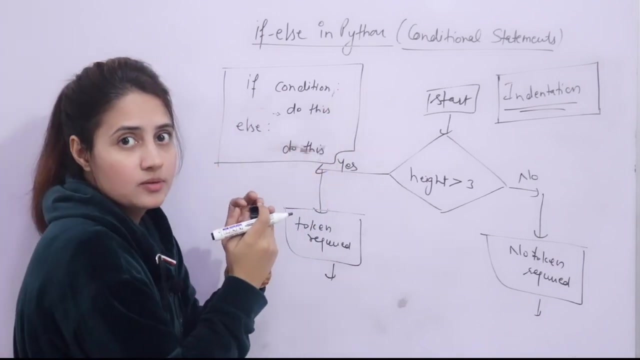 I'll show you, with the help of programming right, what type of error you will get after else. also, you have to do some indentation and here, if we are writing multiple statement, like three statements, so all the three statements should be intended, leave some space here and then write down these statements. 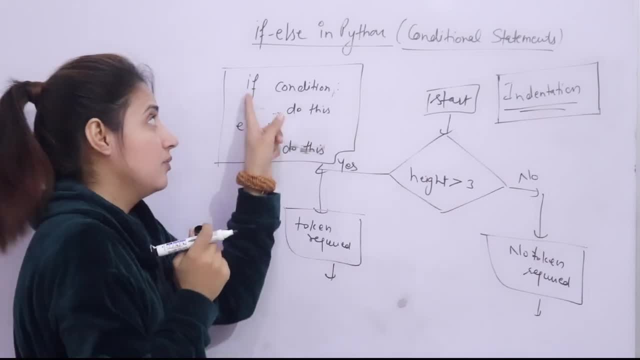 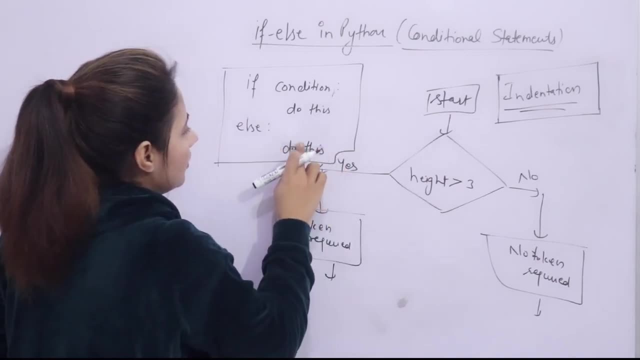 right. so those statements would be considered as block of statement after. if right. so this is general syntax of writing. if now, let me just show you this thing with the help of one program. so this is general syntax of writing. if now, let me just show you this thing with the help of one program. 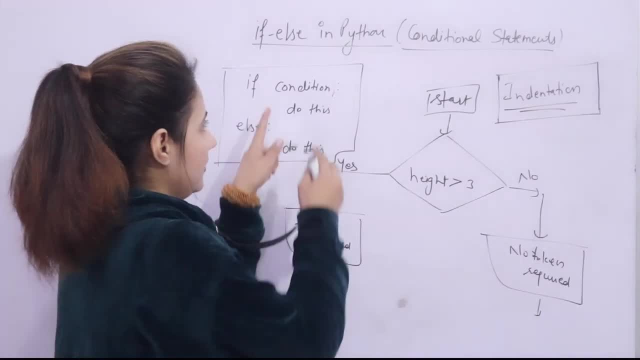 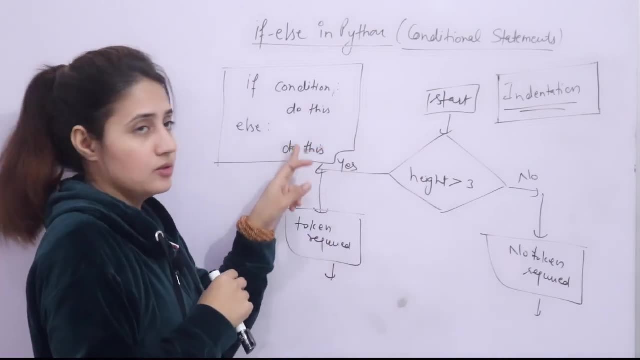 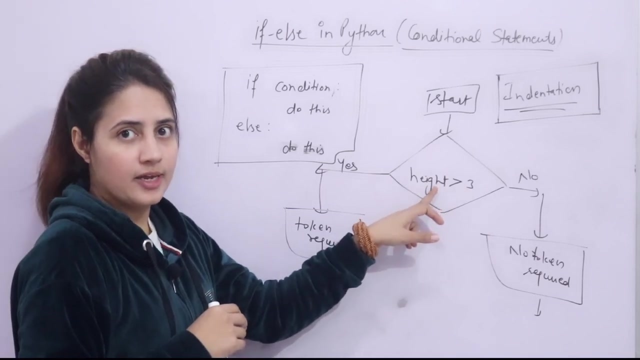 and practically we'll see this thing. so here, obviously, this condition should be evaluated and should return either true or false. based on true or false, this, this the control will go either in this block or in this block, right. so like height greater than 3, so we'll enter height. like height is 4, 4 is. 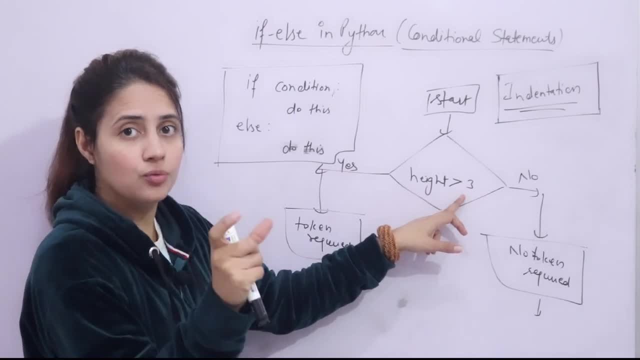 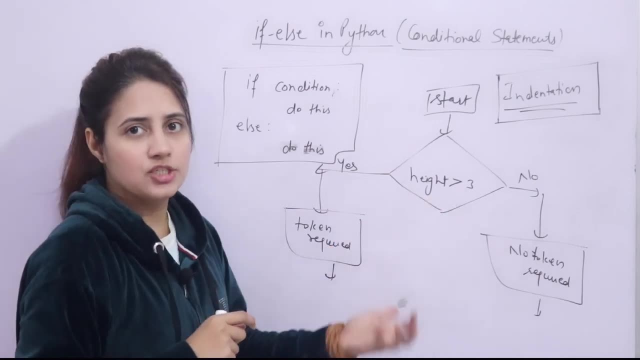 greater than 3 or not. yes, so that will give you, that will give true. so true means token required. yes means this way will go right. so here we are using these relational operands. so we are using these relational operands. so here we are using these relational operands. so here we are using these relational. 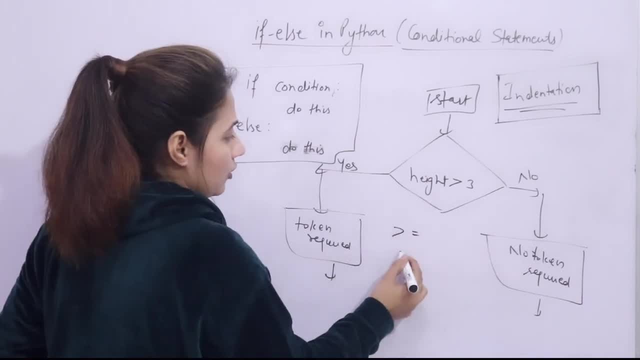 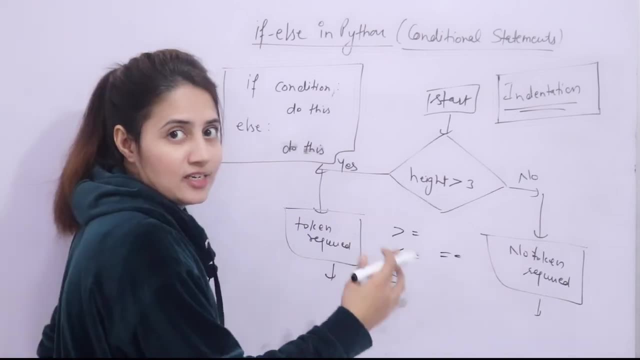 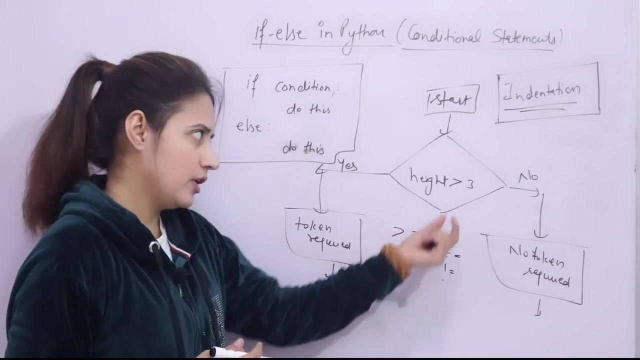 operators or we can say comparison operators. we have discussed this thing: like less than equal to, greater than equal to, or like less than greater than or double equal to like. for equality check we use double equal to or not equal to. these are some relational operators for comparison operators. we 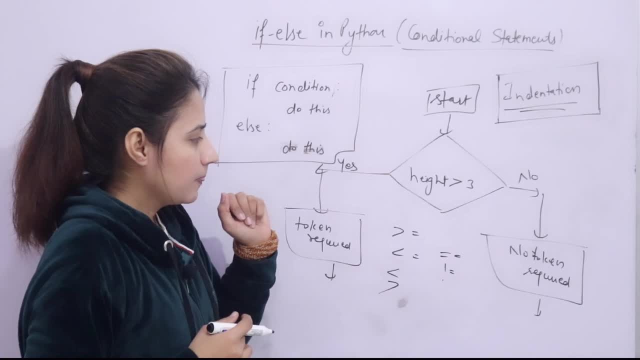 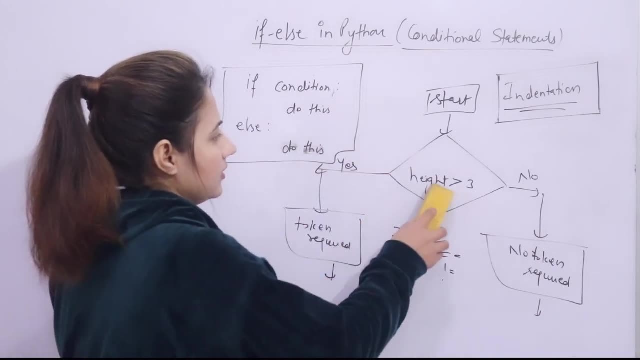 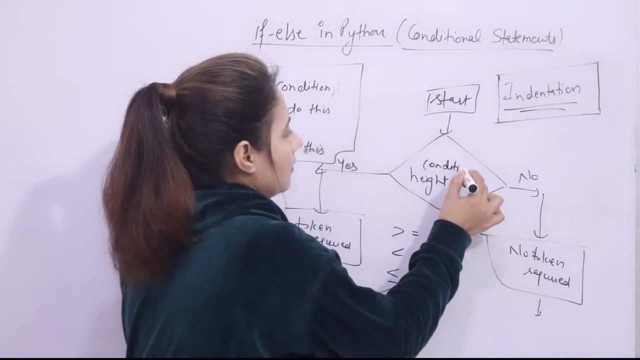 can use while checking some condition, while giving here some condition right now, let's see with the help of one program, if you want to draw general flow chart for this. if else, then simply here we, rather than height greater than 3, we simply write like condition here: condition condition, true, or? 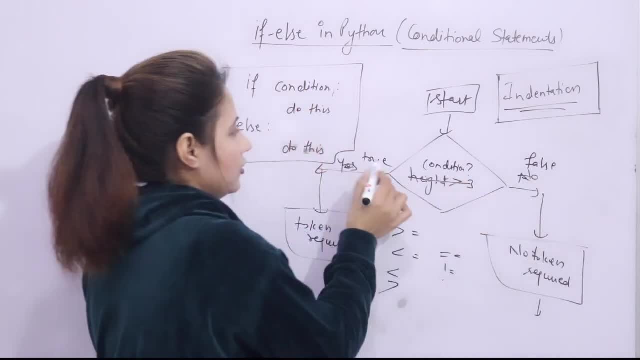 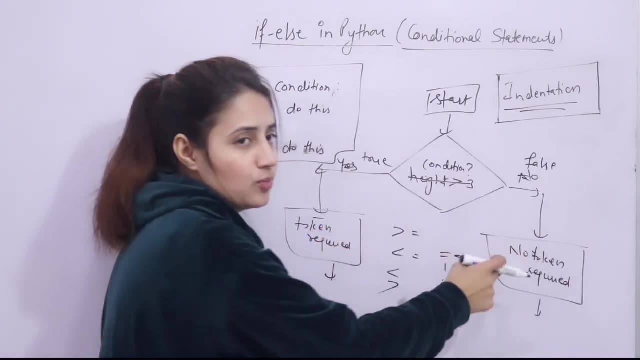 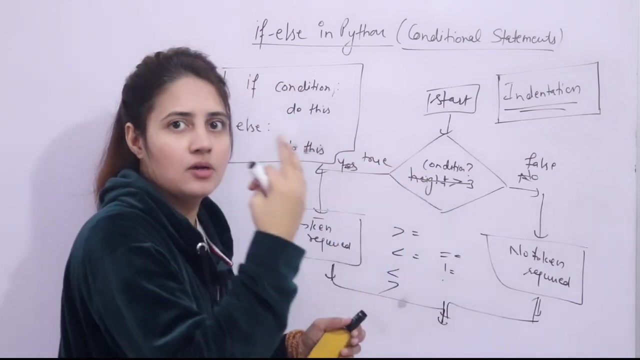 false. two cases can be there: right: no true. true means here we can write if, if block statement, if block statement will be executed here, else block statement would be executed, and after that, obviously program will you know, after whatever statements, after those, if else block that would be executed. 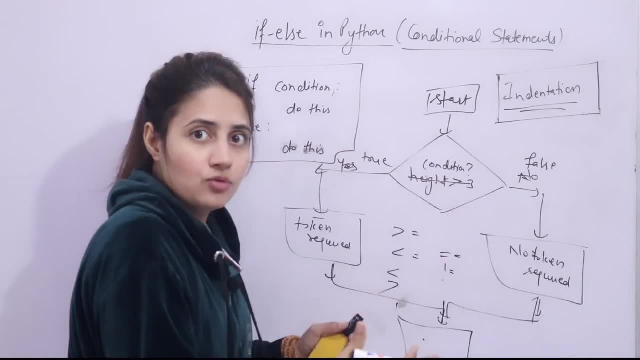 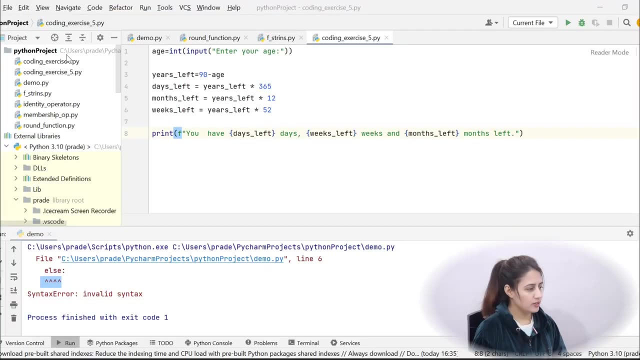 executed right, Right, That would be executed. Statement out of if else block that would be executed Right. So thus you can say general flowchart of if else Right. So let's create a new file and we will be discussing. if else Right, So if underscore. 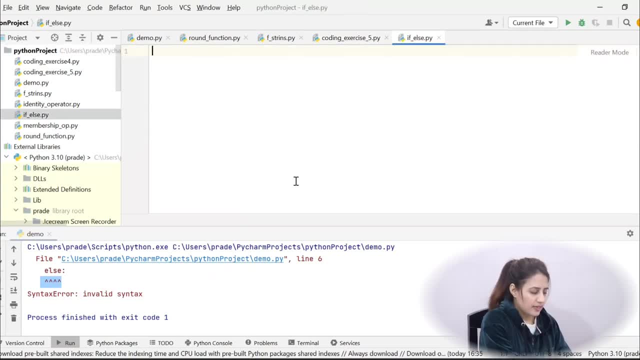 else dot py. Right, Let's take height. So directly, when we are taking using input function, we can convert that into integer, because we know enter height. whatever you will take using input function, that would be string. So convert that into int Right Now let's check what. 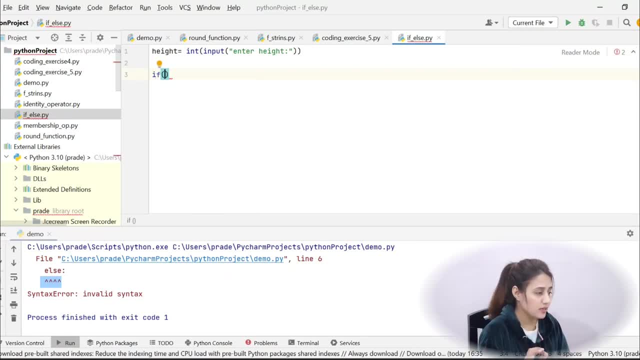 is the condition if height your child height, child cited- is greater than 3 feet. Let me just write down this thing: Enter height in feet Right. So if height greater than 3 feet, Right Column C, As you can see, Whenever the cursor is here and whenever y I will enter. I will press enter, see automatically. 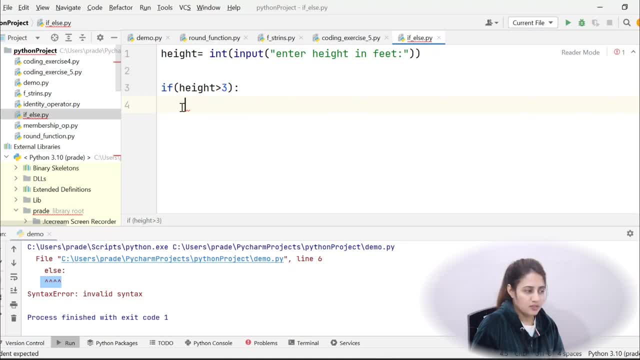 the cursor is here. There are some space in the beginning of this line, So that is what Indentation. That is very important. Then print what we should print. height is greater than 3, then Token required. or we can say by token Right Enter. 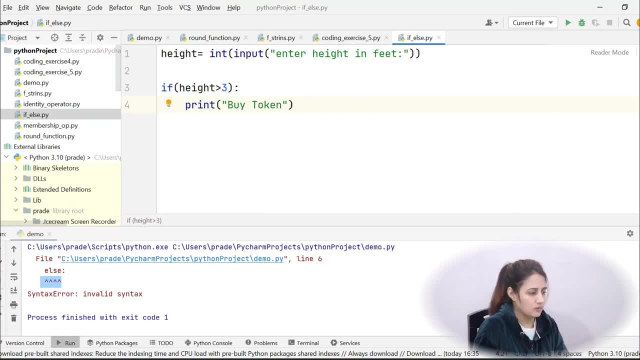 Now else we will write here. no indentation before, else Column C, As you can see. So if height greater than 3 feet Right, Enter Now, else we will write here. no indentation before, else Column C. As you can see, There are some space in the beginning of this line. 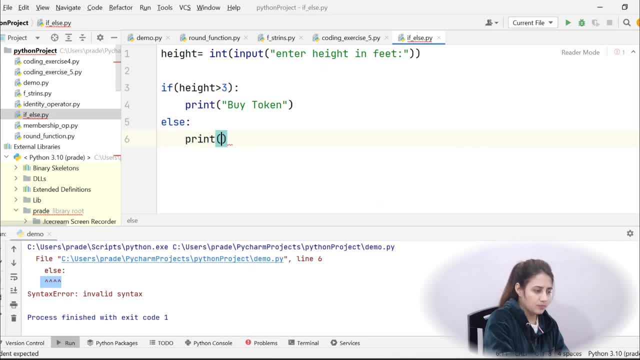 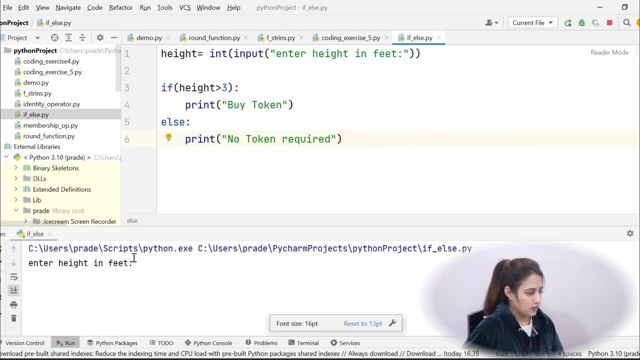 There are some space in the beginning of this line. So that is what Indentation. That is very important. Then print what Indentation anotherí And print no token required, Right, Okay, Letís run this and I will show you. first of all see, It is asking: enter height in. 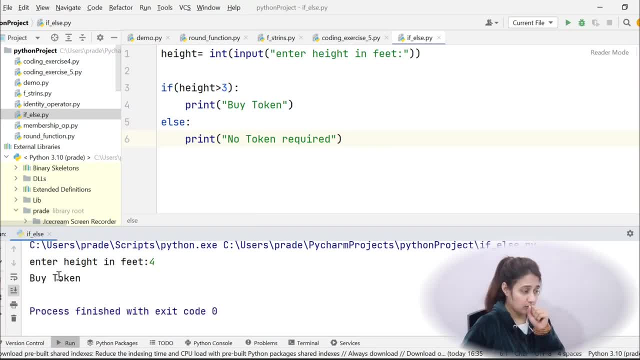 feet, I am entering 4.. So by token, because height is 4 greater than 3, this condition is true. So control will enter here and by token, Right? If I again run this and I enter, then no token required because condition is not true in this case. so control will go in else part. 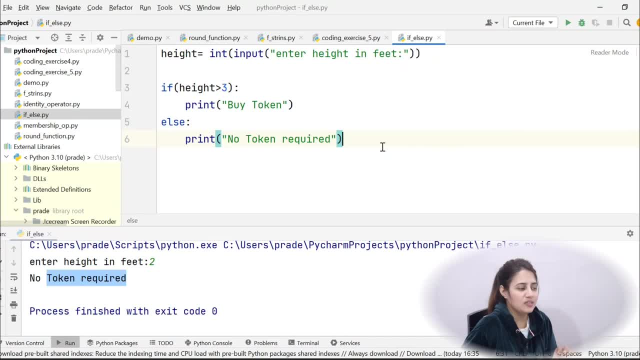 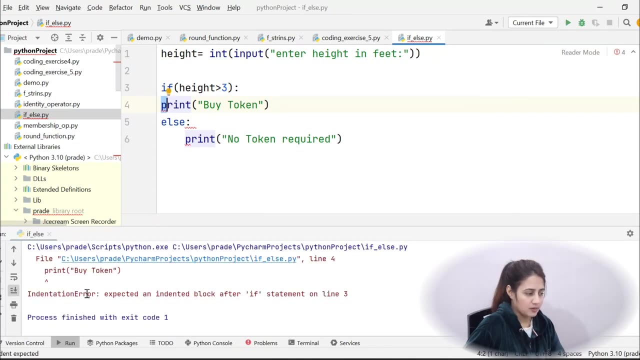 and no token required. so this is simple working of if else statement. now let me just show you something: if you do not now put here that indentation or the white space, then see, you can see this red line here and let's run this. see this, there is something wrong here, because this: 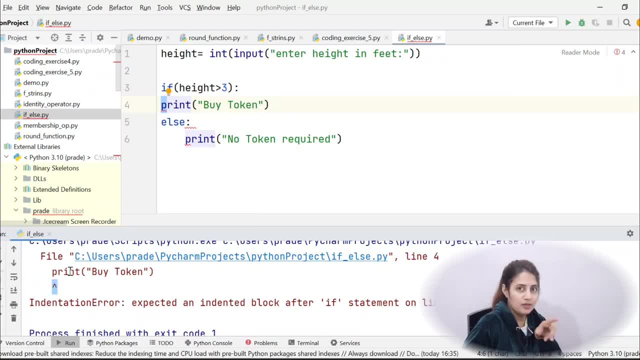 this is some arrow. there is something wrong here, so it will give you clue. and error is indentation error. the error name is: this: is indentation error, expected and indented block. after if statement on line number three. so after if there should be some indentation, that is indentation block. so 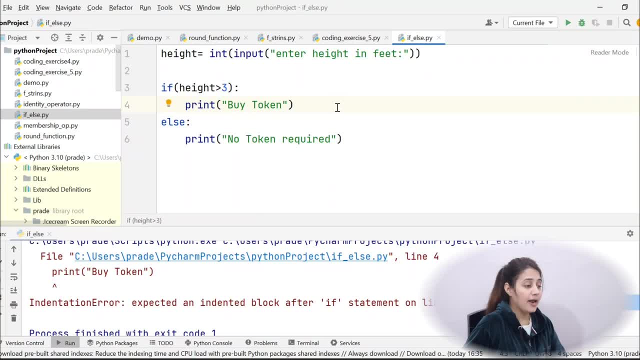 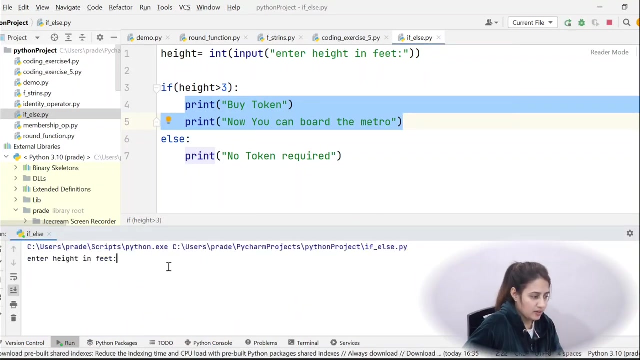 that should be indented. and if i write one more statement like print: buy token, token and now you can board the metro, right, so see these. both these statements are intended right? so this would be considered as a complete block, block of statement after. if so, now, if i run this and if i enter height, 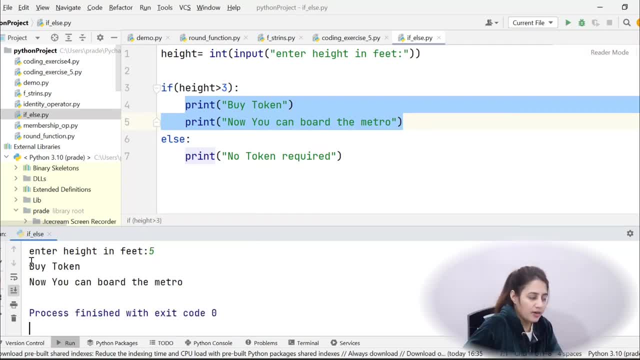 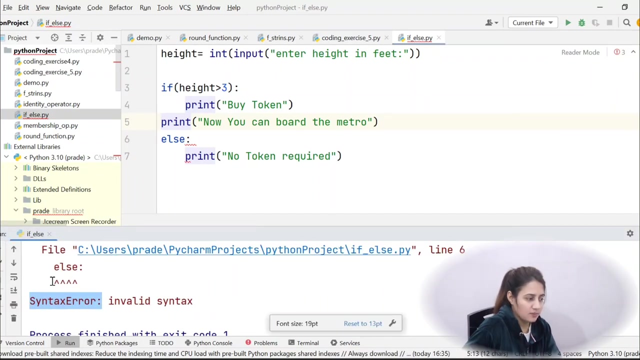 like five. so and now you can board the metal, these two print statement would be executed, because this is now block of statements. after if, right, but after this: if i do not put any indented indentation, it will give error. let's run this. see syntax error. this is syntax error, something here in else part, because 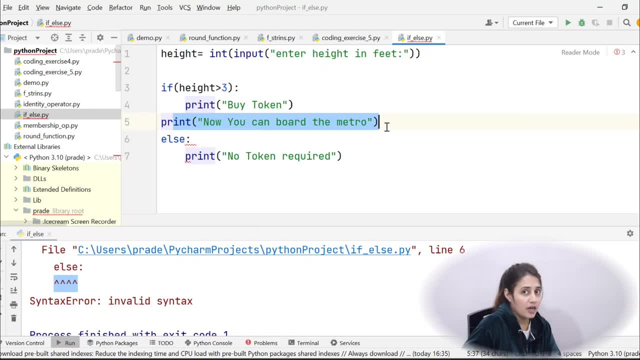 between if and else. this print statement would not be considered now as a part of this if block right. but if you are using if else, between if and else, there should be nothing right and you are writing this statement, so this is wrong. better, you put this in this block right. so i hope you got this thing. how to use if else. now if simple if rather than 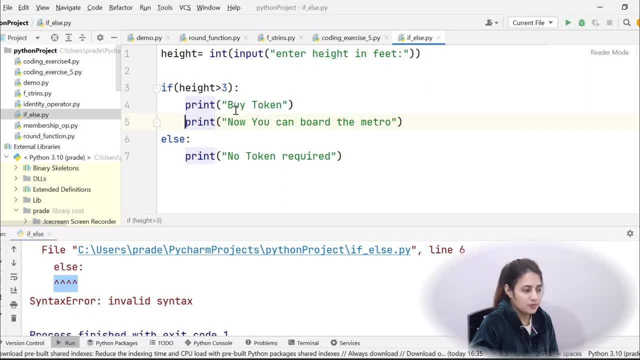 else we have only one choice, simple: if right, no else part. let's suppose, remove this else part, comment this out. and if height is greater than three, then by token, and this thing, that is only case, no else part. let's run this. greater than three means six, so by token now you can vote the metro, and if this is less than three, 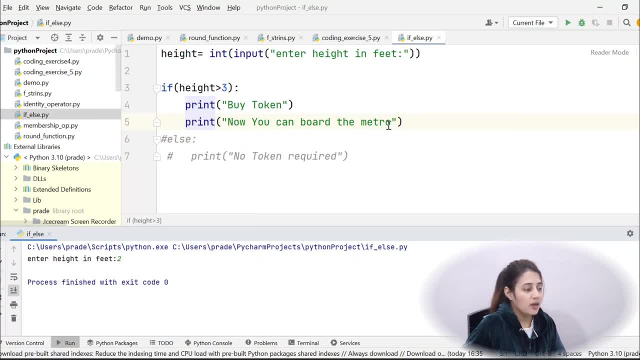 like two, nothing would be printed because there is no else part. but but if i write one more line, something like this: print out of if block. this statement is out of if block because there is no indentation here. let's run this and height is now. i'm entering two, so now it will print out of if block this. 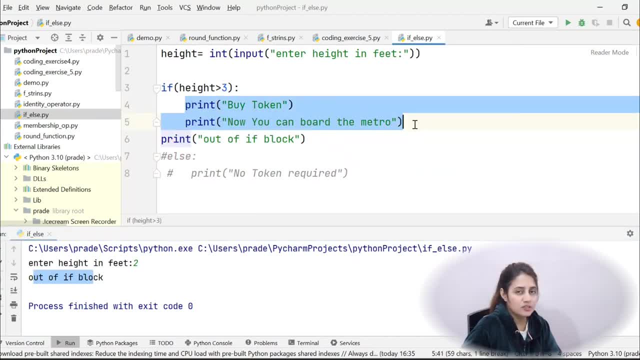 print statement only because these two print statement would be considered as part of this if, because these are intended, this is not intended, so this is out of it if i do not put any indentation here. so now this only would be part of this. if block. these two are not part of if block. 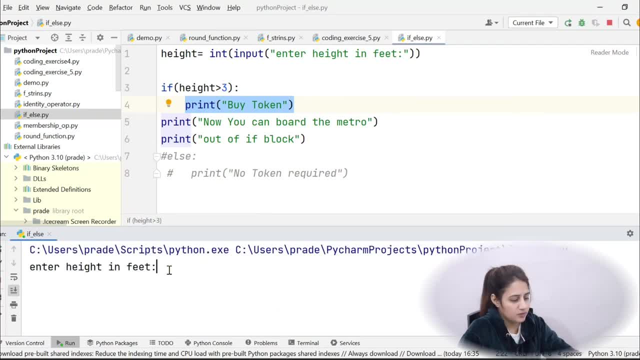 let's run this: and if i enter six, so height is greater than six, is greater than three, so only one line would be printed by token. that's it right? sorry, by token. and now there is no else part. so these two statements are part of program only so obviously after if those statement would be. 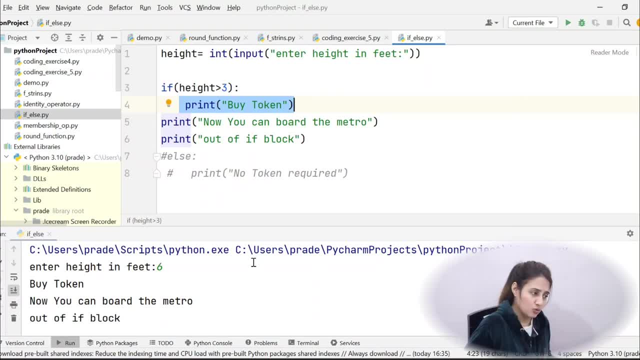 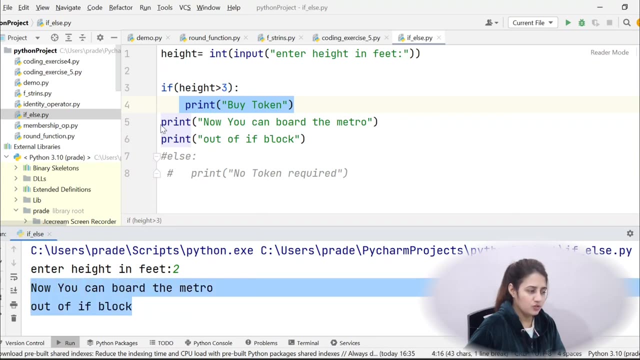 executed that are part of program. normal execution of program would be there. so these three statements would be executed right. and if i run this and if i enter like height is two, now only two statement would be executed. now you can vote the metro and out of if block these two only because now this 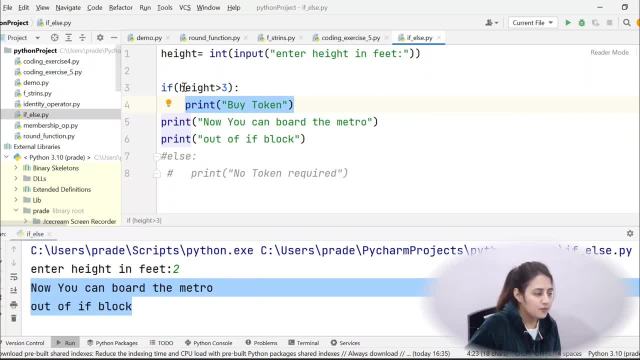 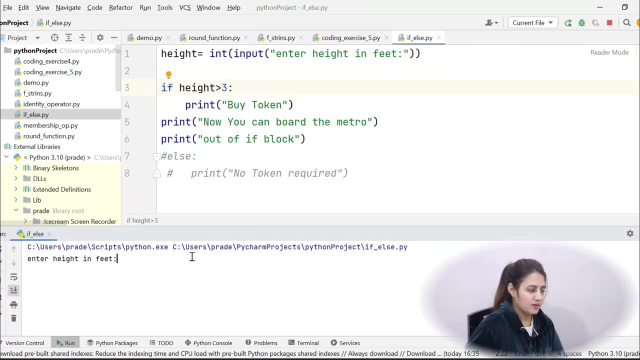 print by token is part of this. if block right and if you do not put like these con, sorry, the these brackets, that is also fine, because i am actually from c and c plus plus background, so that is why i used to put these brackets. let's run this, there would be no error. right, height is three, if i. 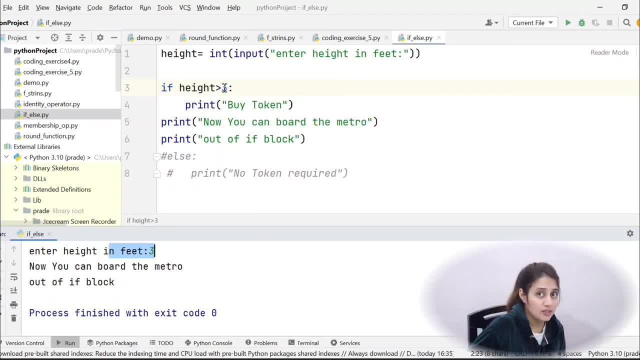 enter height three, because three less than three no condition is not true. so now, no, if block these two, statement would be would be executed. right, let's do this thing and let's comment this out, and if you want to put that condition also, like if your child 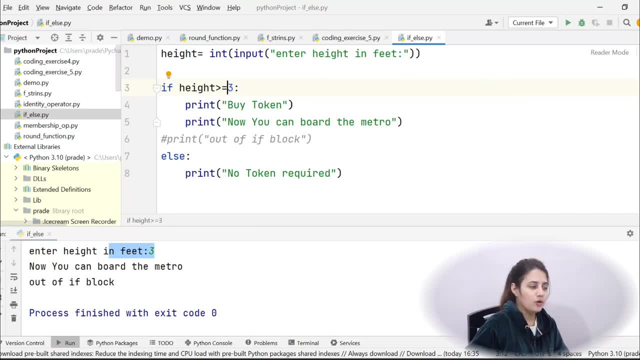 height is greater than or equal to three, then you have to buy token. less than three, then you need to buy. so less than equal to, greater than equal to this, and you can put. or if double equal to you want to check equality, then double equal to, also we can check. 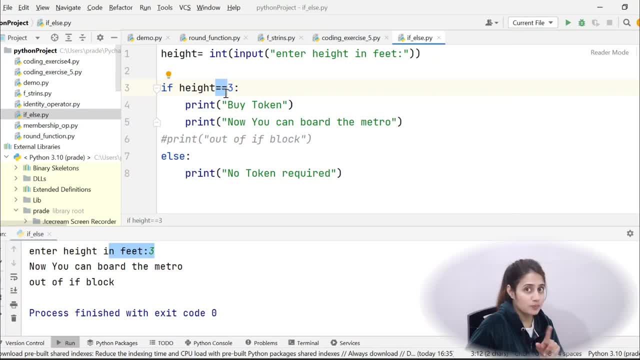 but for equality you have to use double equal to, not single equal to. that is not. that would be. so there would be some some error, like if i put only one, one equal to. i want to check equality if height is equal to three, but i only put one equal to, so there would be some error. let let me just run this. 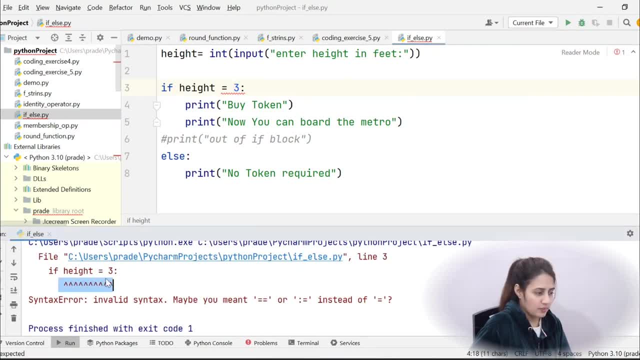 and see it is showing here are some error. if height is equal to syntax, error invalid syntax. maybe you meant double equal to for this instead of this. so it is giving you some clue for this. so it is giving you some clue also. you can read out these error and you can check where is the error. 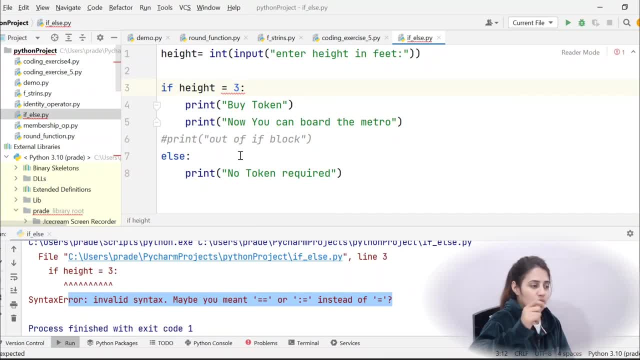 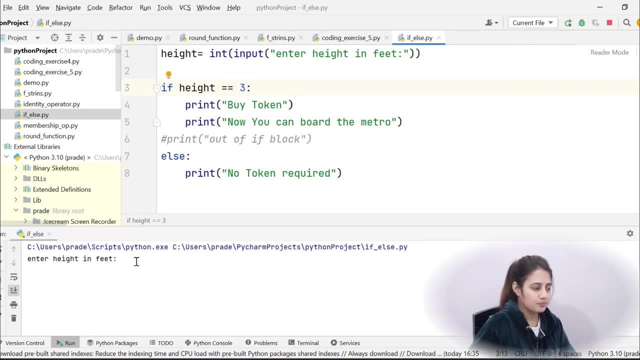 so here should must be some error. so maybe it's not not equal to a double, double equal to. it should be double equal to now it is. there would be no error, right? if i enter height four, then no token required, because condition is not true. height is not equal to three. 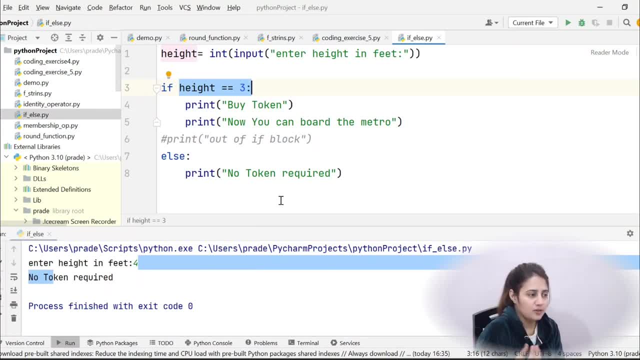 right. so i hope now you got basics of if and if else statements and how to use them and what is indentation and how this indentation is important. If before this height, before writing this, if we put space, see here also in Python it will give error You cannot put.